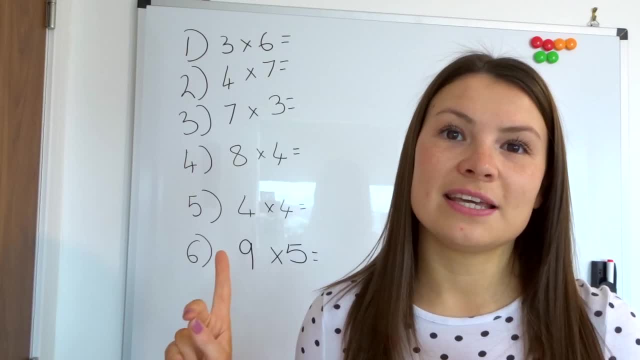 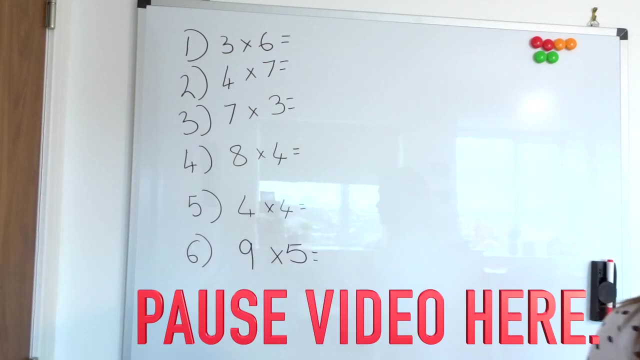 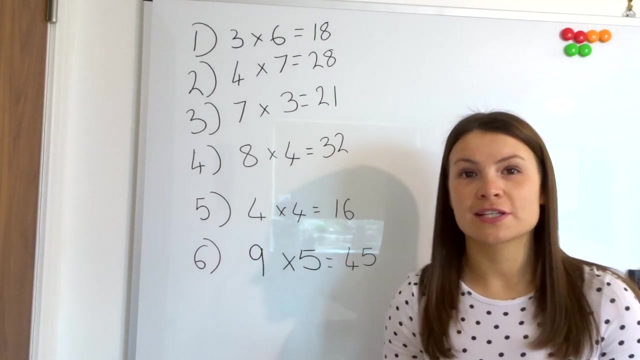 board here. So just quickly have a go at doing these, work out the answers to them, and then I will be back with you in just a moment. So let's get started. Okay, and here are the answers to those questions. So now go through the work that you've just done. 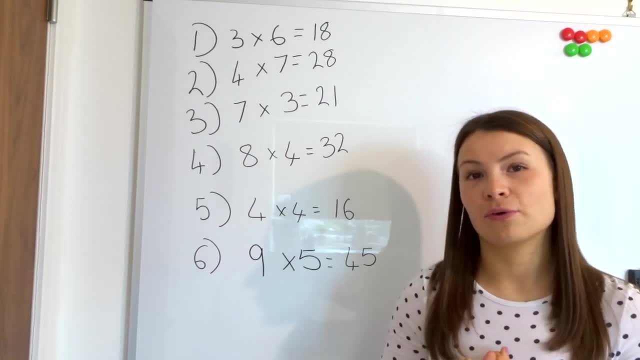 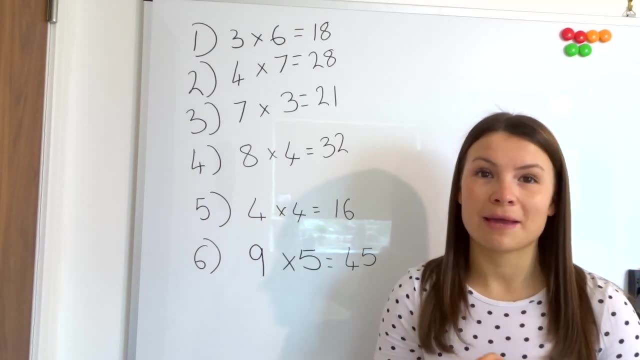 and give yourself either a tick or a dot for where you've got them correct or where you have made a mistake. If you have made a mistake, just go back and just check where you made that mistake. So, like I said, we are going to be looking at written method for multiplication today. So the first 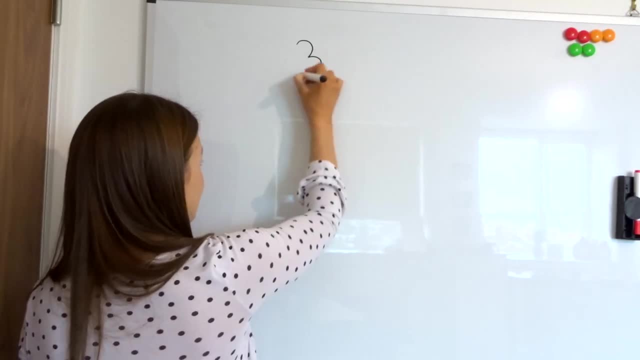 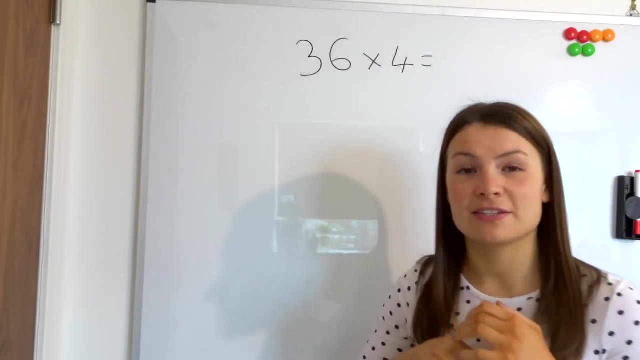 question is: what's the most common Prose粒 number of a number? The answer is 36 times 4.. So 36 times 4.. Now for a few of us looking at that, that might seem really complicated and like we can't do it. 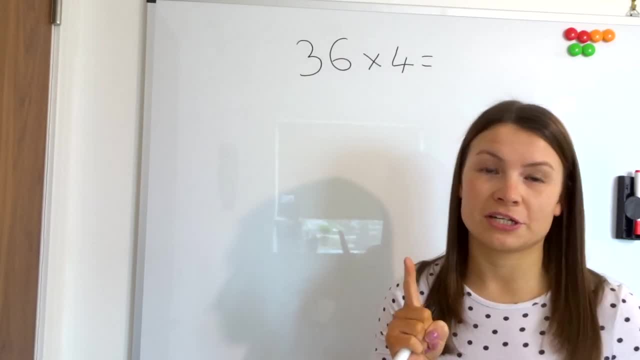 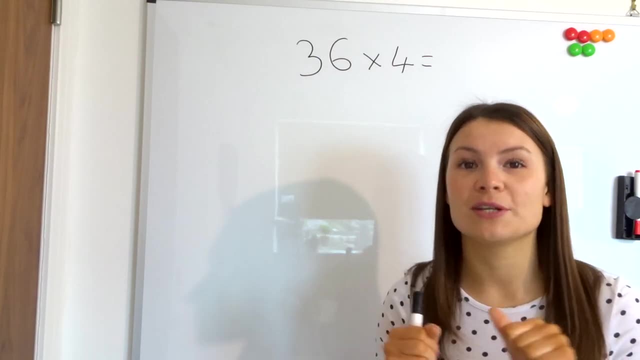 because we are timesing a two digit number by a one digit number. Now, that is different from what we are used to, because normally we just do a either one digit number by a one digit number or we do a two digit number that's not as big as that by a one digit number. Okay, so now let's get. 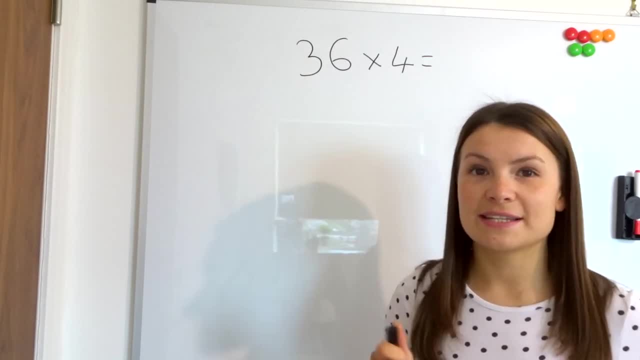 back to that one. Okay, we have got our first question and now we have to figure out the questions. So what are your answers for this one? So what we are going to do is we are going to. So the written method for doing this is really similar to the way that we do the written. 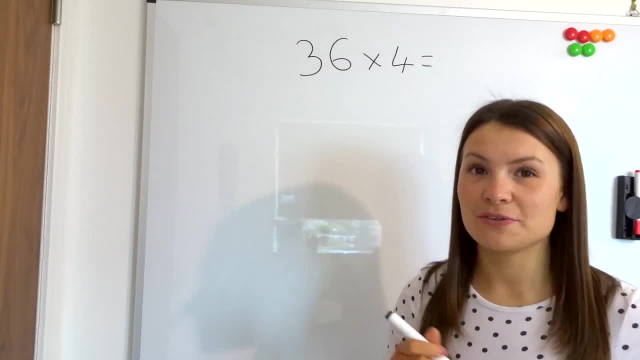 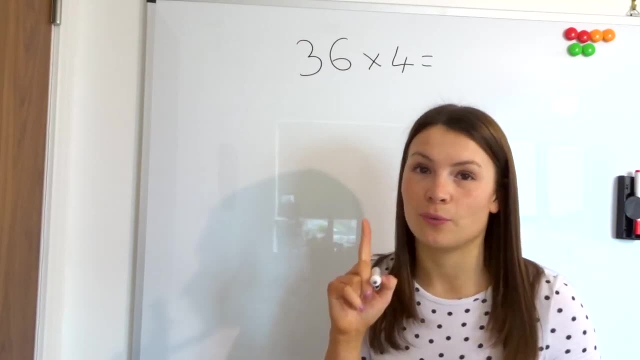 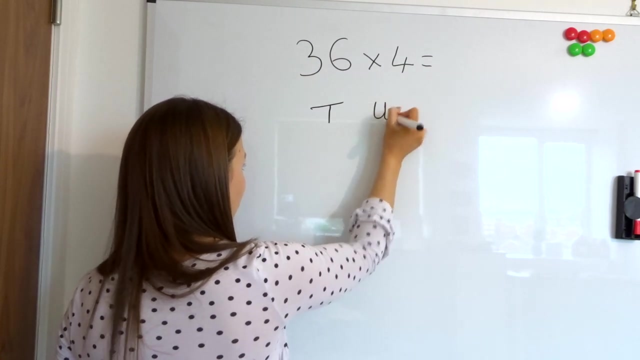 method for addition and subtraction. So we do lay it out with our hundreds, tens and units column. So we haven't got any hundreds in this number here, but we have got tens and we have got units or ones. So we've got tens column and I'm going to call it our units column. 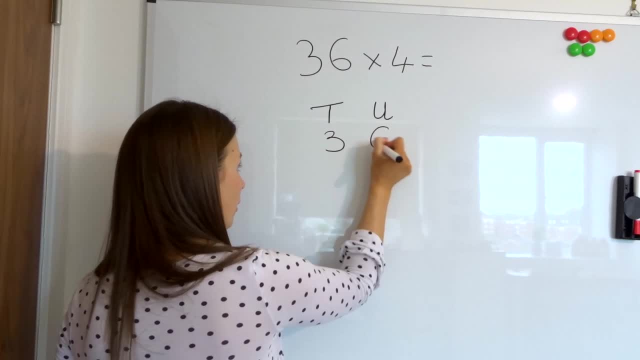 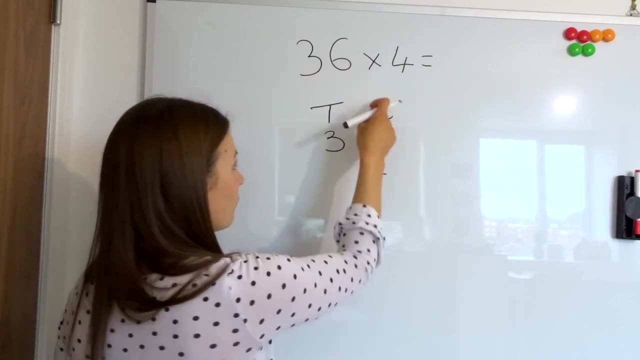 So we write 36, because we put the biggest number on the top and then we put the four underneath the six. So we've got 36, which is the biggest number, and then we've got the four in the units column, which is just below. 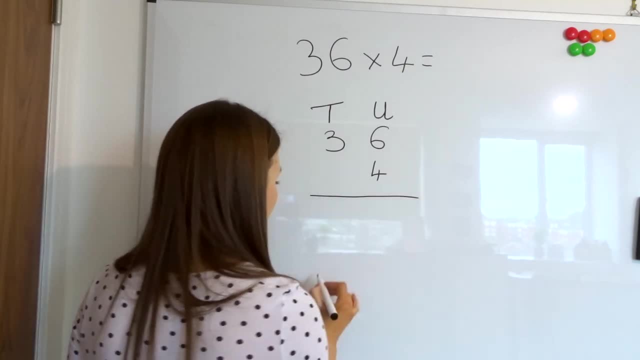 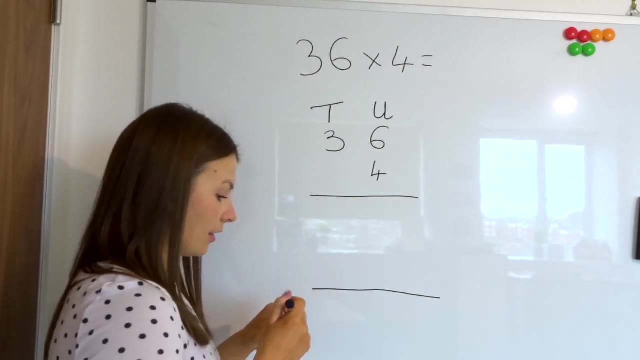 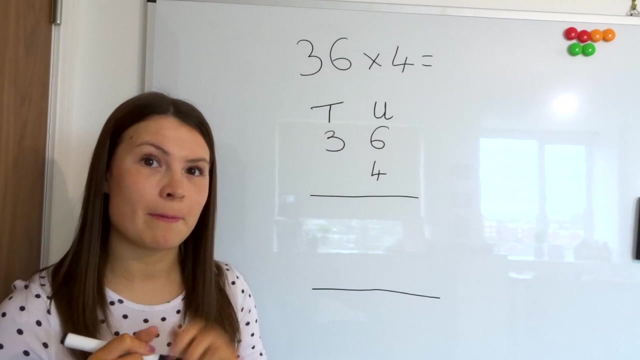 And then we draw a line just underneath and then one a little bit lower down, because we need to get two numbers in here. Okay, so we're going to start off. oh, I've missed something off. Can anybody tell me what I've missed off? 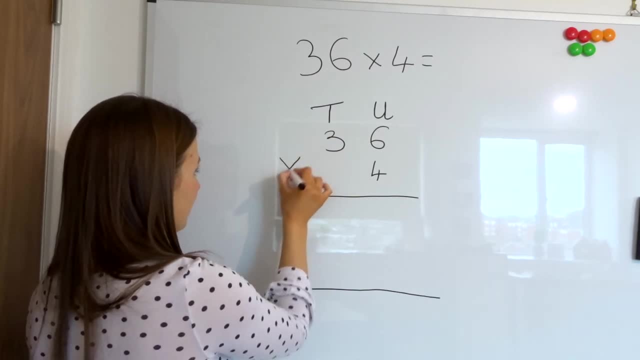 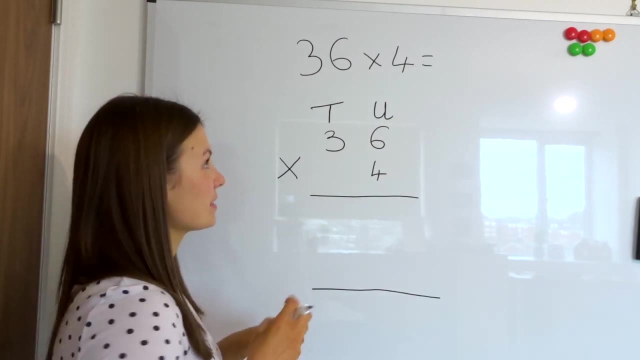 That's right, I've missed off the multiplication. Okay, I've missed the multiplication sign here, because we need to remember that we're multiplying, not adding or subtracting. Okay, So we're going to start off by timesing our units column. 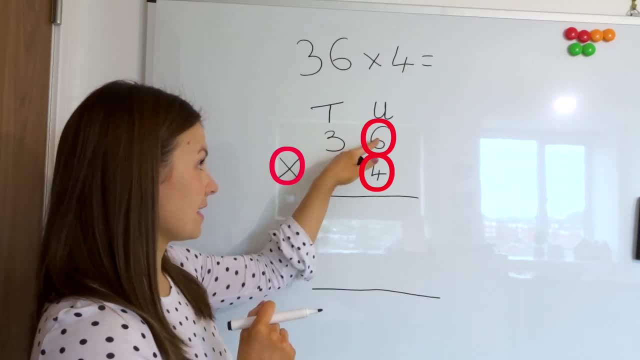 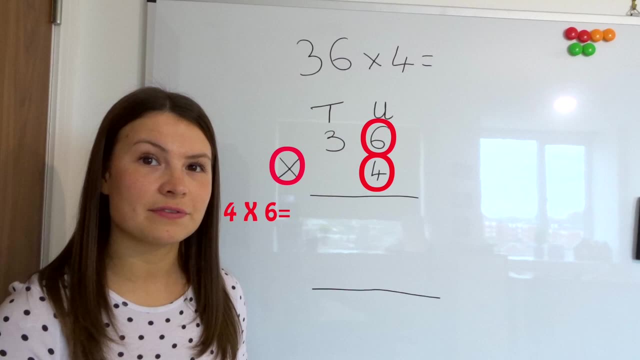 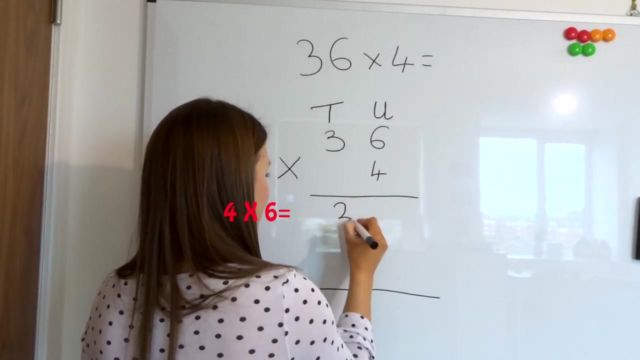 So we need to do four times six. four times six. work that out for yourselves. Okay, You are right, It is 24.. So we are going to put 24 and we're going to write it like that. Fantastic, Okay. 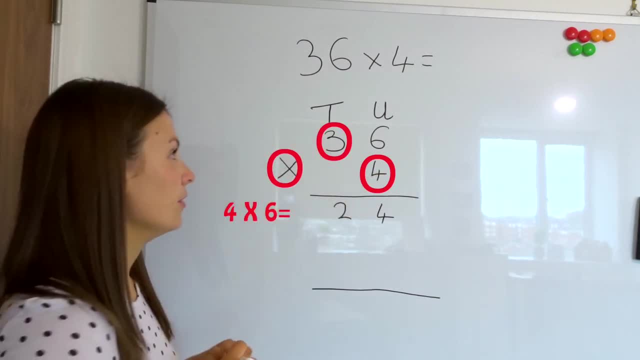 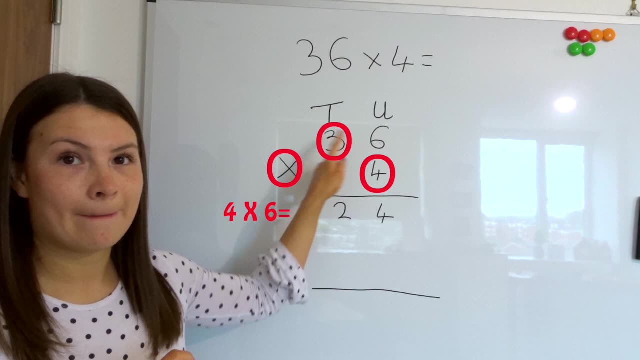 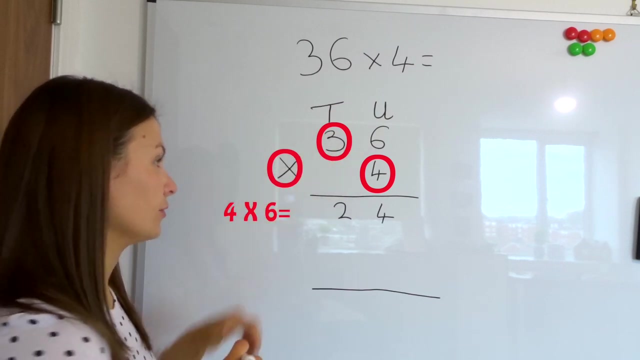 And then we need to do 30 times four. Who can tell me the reason why this is 30 and not three? You're right, It's because it's in the tens column. So this number here is actually 30, not three. but for now we can just make it 10 times smaller. 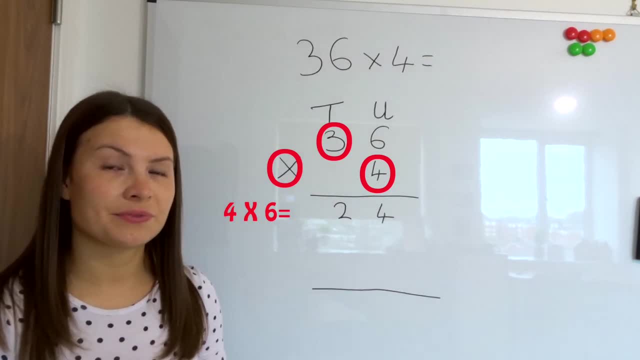 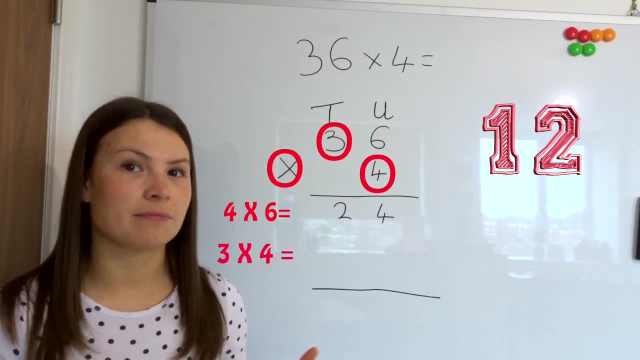 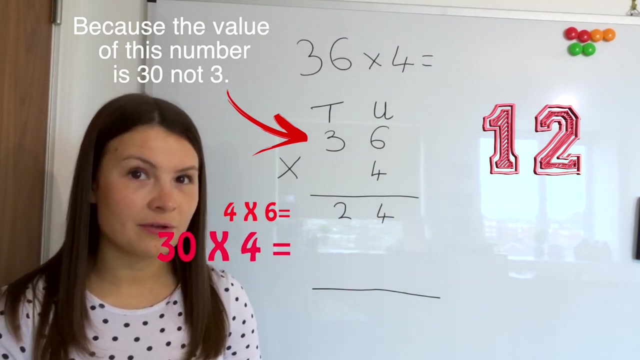 and do three times four. So three times four is 34.. Okay, So that is 12.. Fantastic, But now we need to make that 12, 10 times bigger. So if we're going to make 12, 10 times bigger, what do we get? 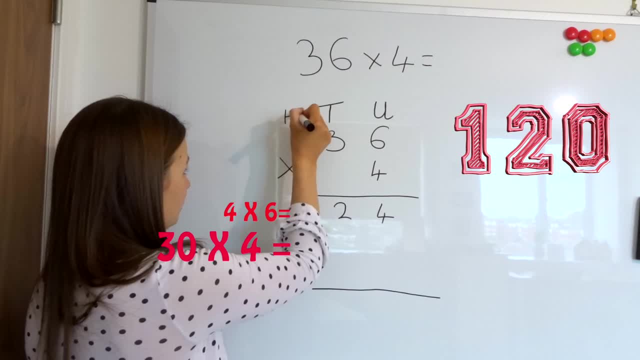 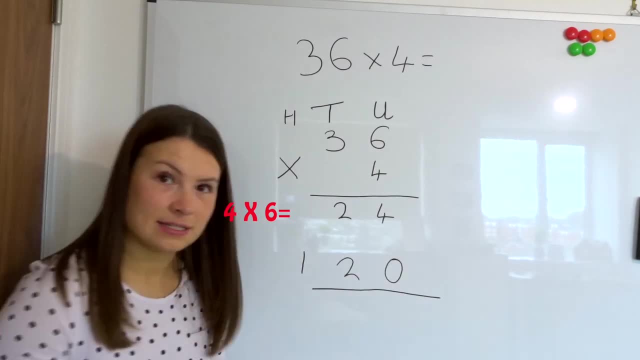 Fantastic, 120.. We've got our hundreds column over here, So 120.. Fantastic. Okay, Now we need to add our two and a half. We need to add our two answers together, because we haven't actually got an answer yet. 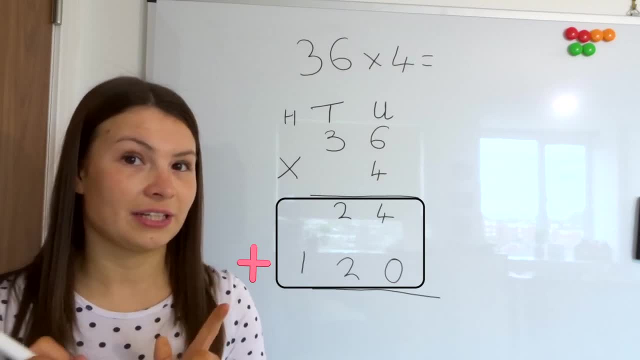 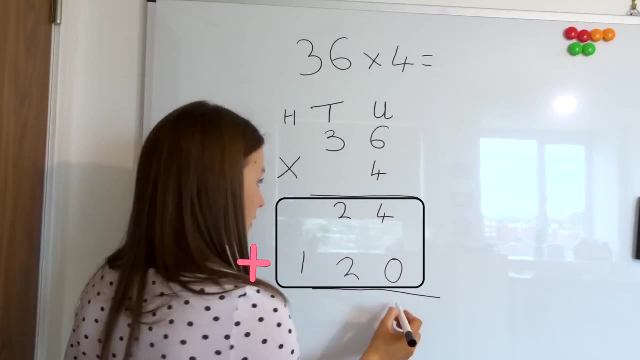 So what I'm going to do is I'm going to use the written method for addition here. So I'm going to start in my units, column Four: add zero- is that's right four, And I'm going to go to my tens column. 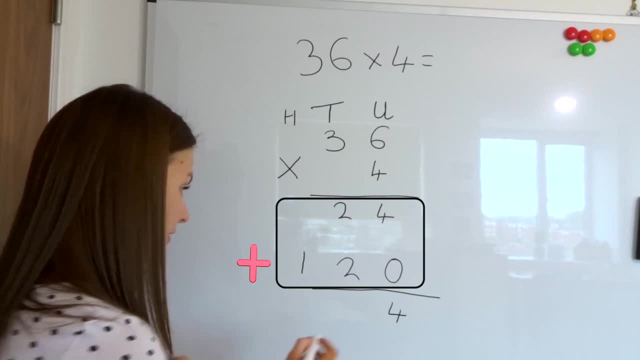 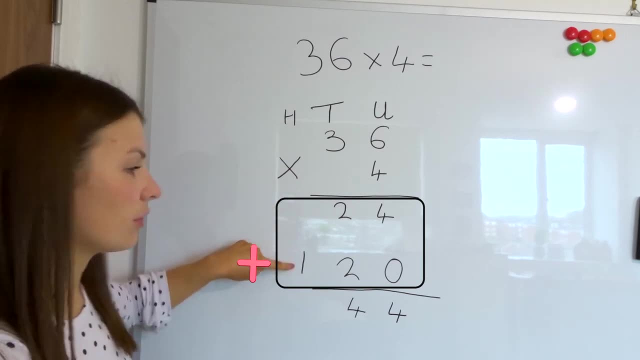 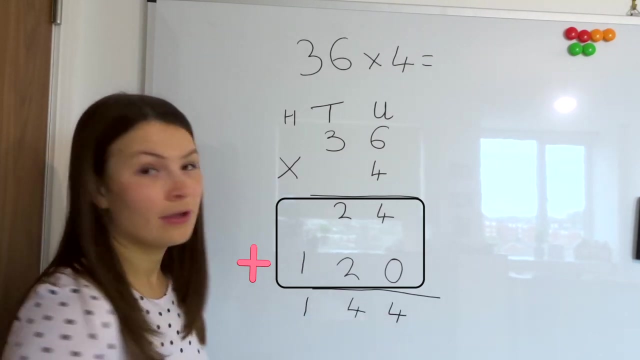 Two add two is again four, And then we're going to go to our hundreds column. We've got nothing up here, and then we've got one here. Fantastic. So our answer is 144.. Great, Well done, Okay. 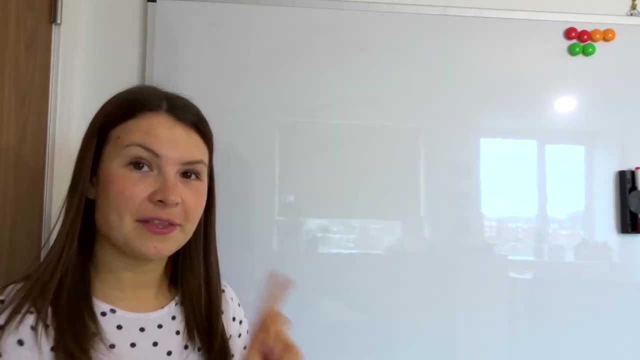 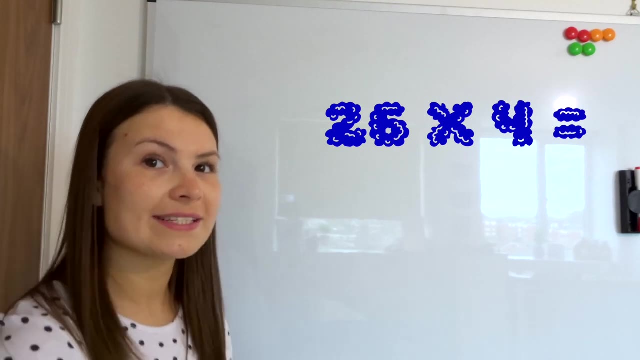 So we're going to do one more with you, and then I'm going to give you a few to do on your own. So the next one we're going to do together is we are going to do 26 times four. 26 times four. 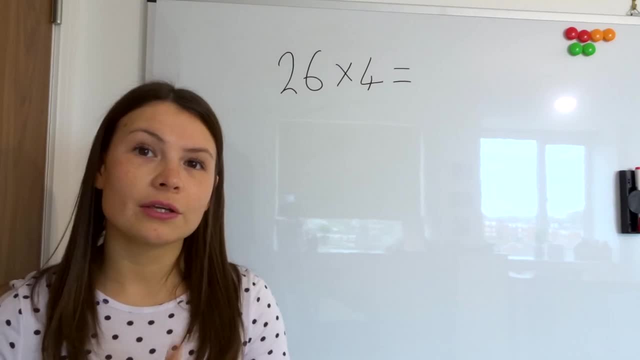 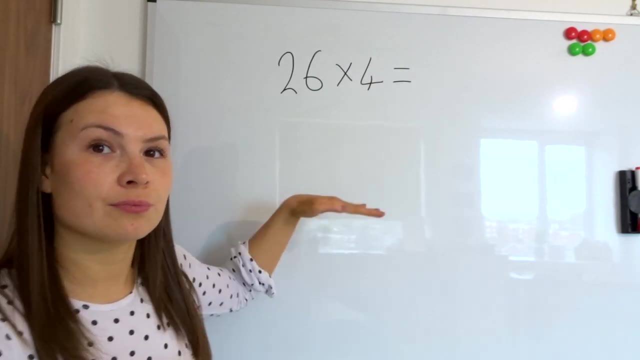 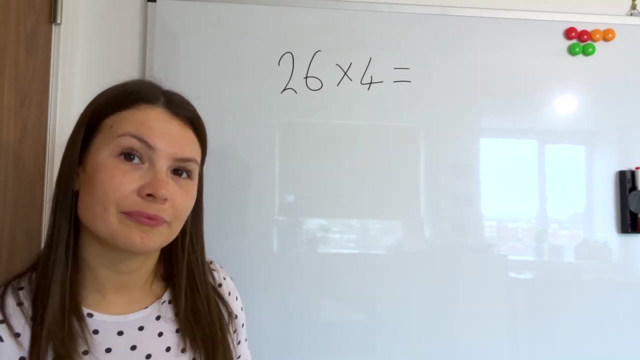 26 times four. Okay, I would like you to write this out in the written method form That we have just learned. So your biggest number on the top and then your smallest number on the bottom. Don't forget to put your tens and units at the top. 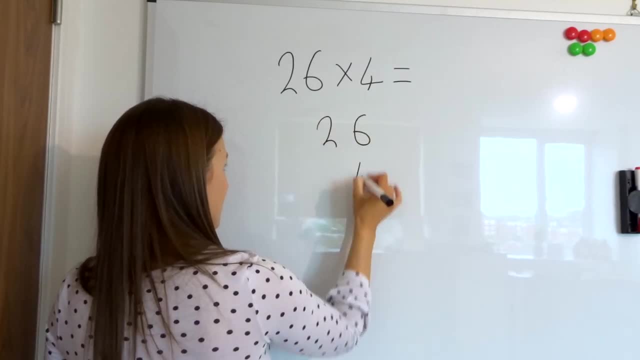 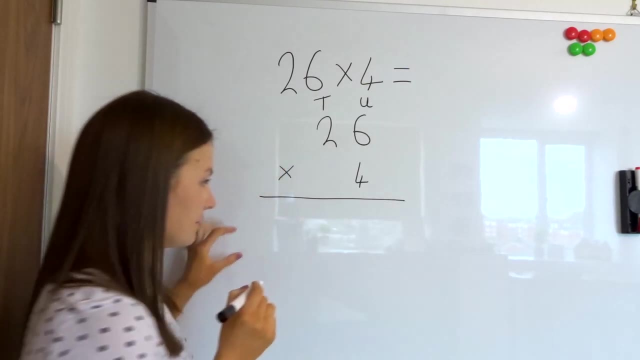 It should look like this: 26.. And don't forget to put your multiplication sign over here. Then we draw a line here, And then we draw a line here And then leave space for two numbers, remember. And then a line here. 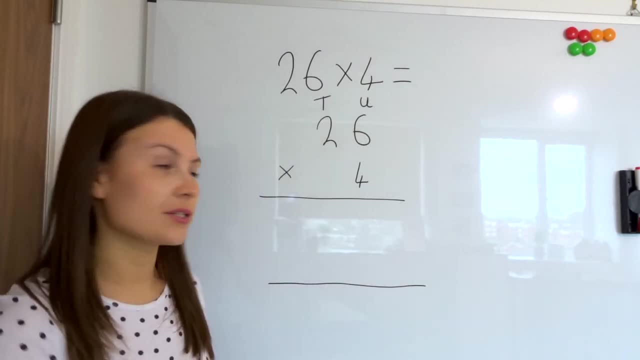 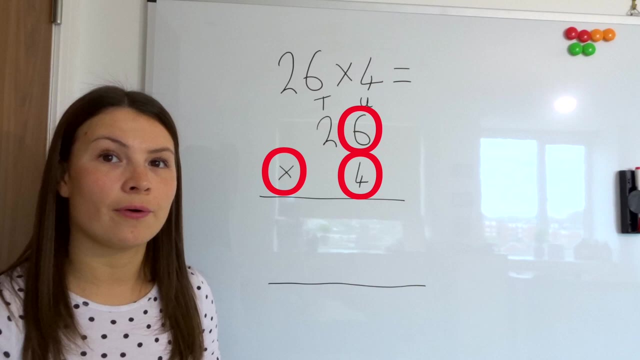 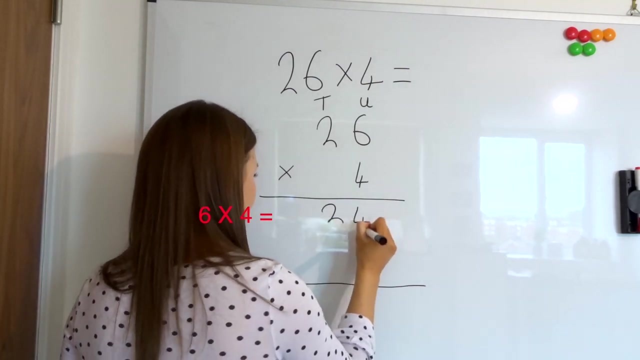 Fantastic, Okay, So we are going to start off with our units column. So six times four, What is six times four, 24.. Fantastic, Well done, Okay. Next one. So we're now going over to our tens column. 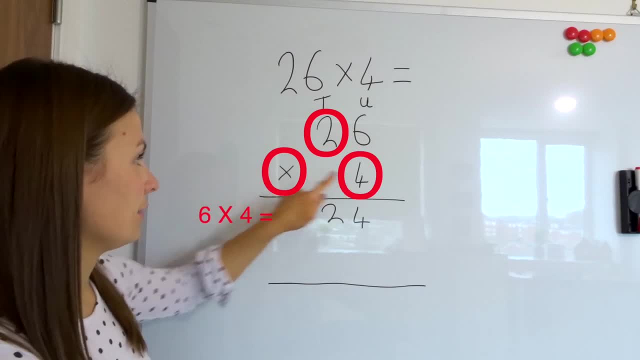 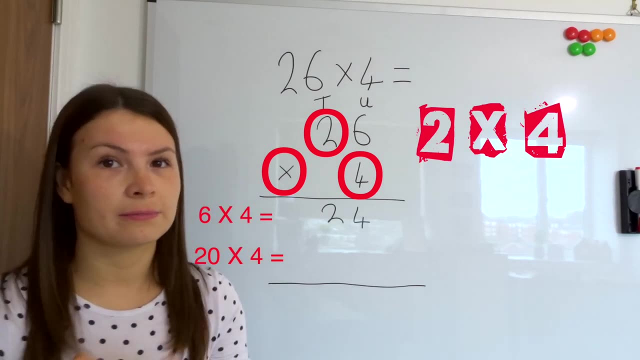 So we're going to do 24.. We're going to do 20 times four. 20 times four- Oh, that's a bit tricky. So what I'm going to do is I'm going to do two times four, And then I'm going to make it bigger. 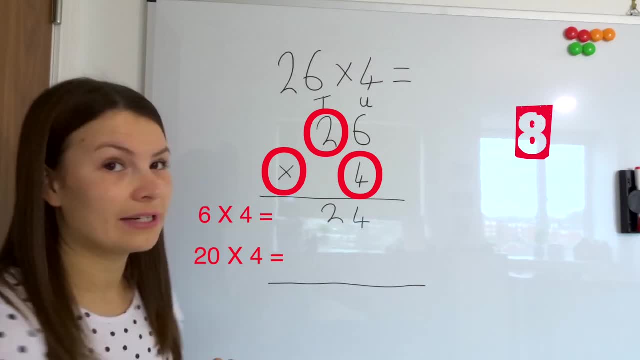 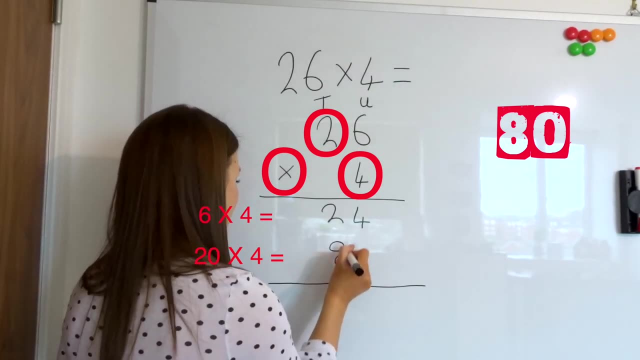 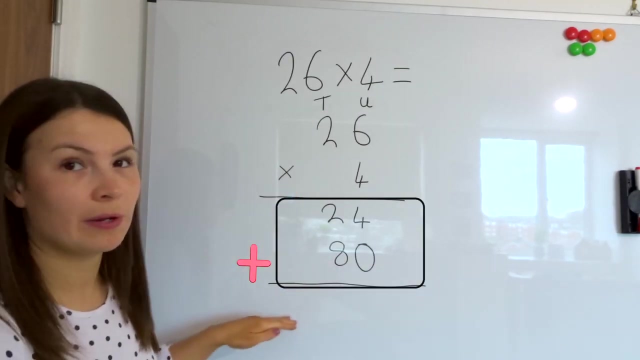 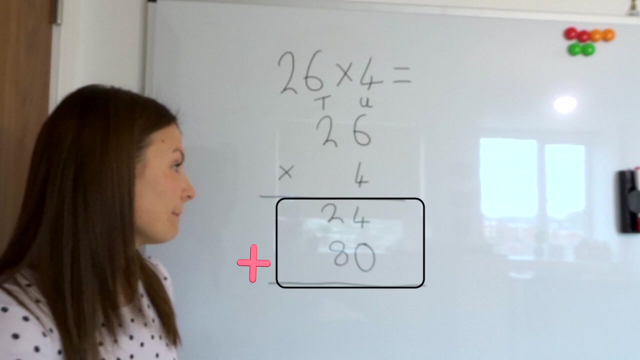 Two times four is eight. Good, Now I need to make it ten times bigger: 80.. Fantastic 80.. There we go. Now I would like you to add these two numbers together and write it just below this line. Off you go. 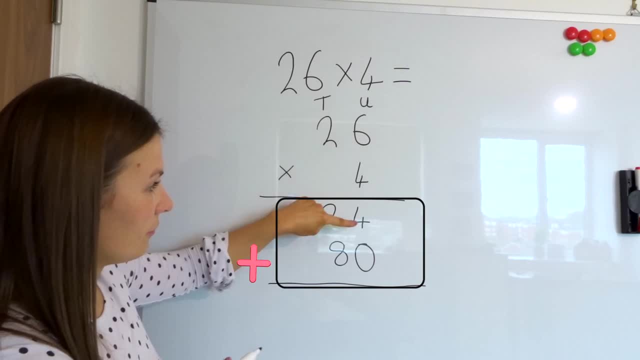 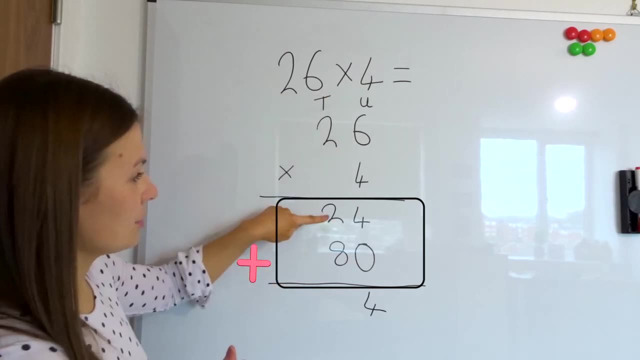 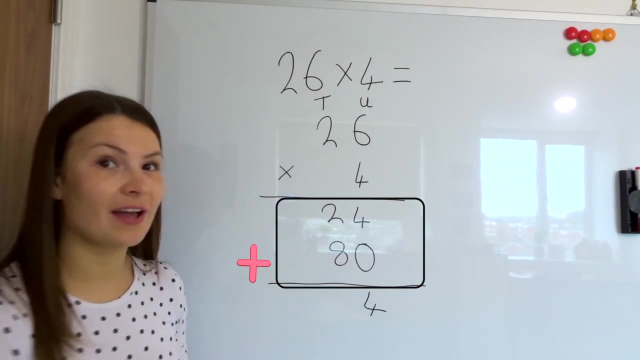 We're going to start off with our units column. So four add zero is four. Then we're going to go to our tens column. Two add eight, Or 20 add 80 is 100.. So the way we write that we put the one in the hundreds column. 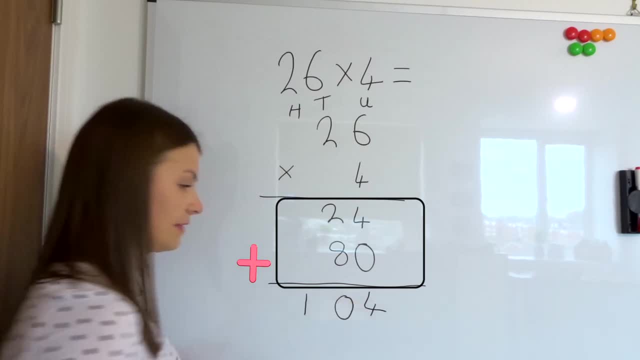 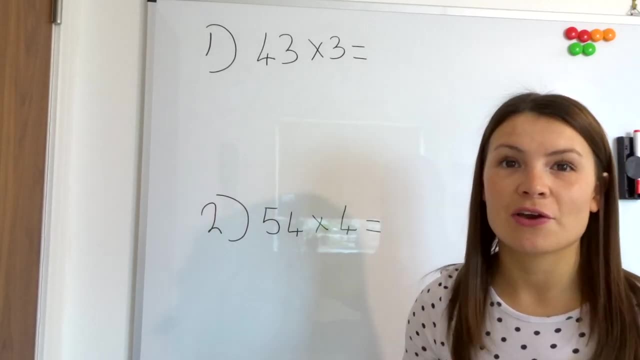 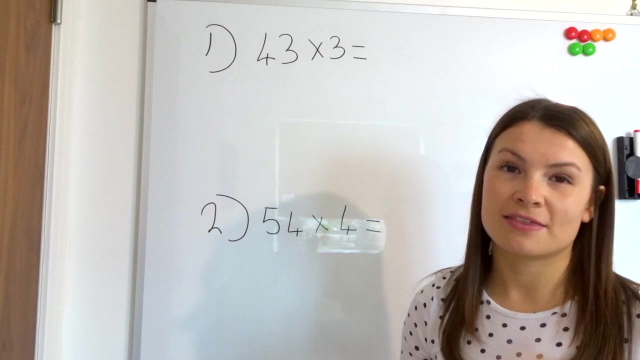 And then we've got no tens- Fantastic, So the answer is 104.. Well done, guys. Okay, So now it's your turn to have a go at doing some of these on your own. Pause the video here and have a go at answering these on your own using the method that I've. 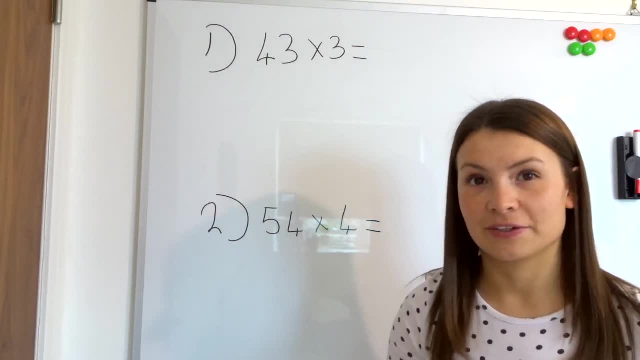 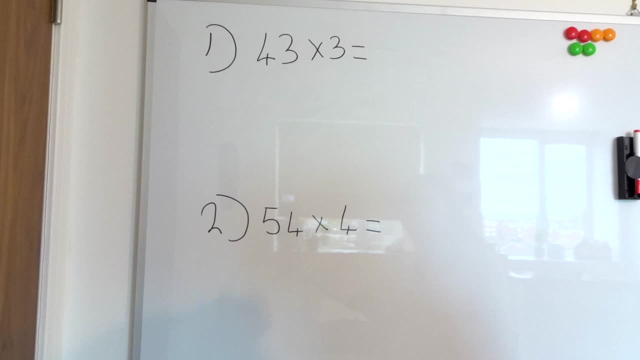 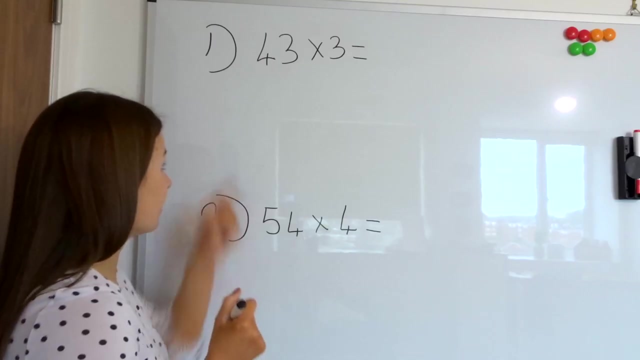 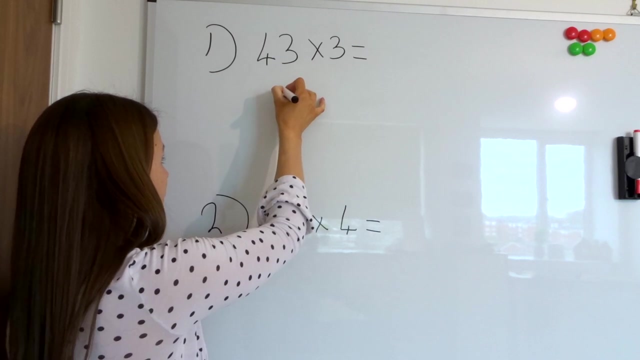 just taught you And I'll be back with you in just a second. So let's start off with number one. So we've got 43 times three, So we're going to put our biggest number on the top, So 43.. 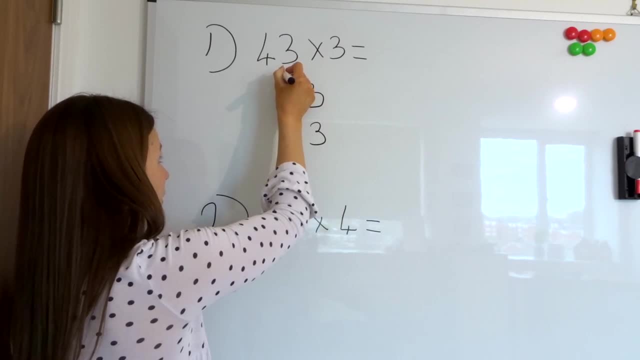 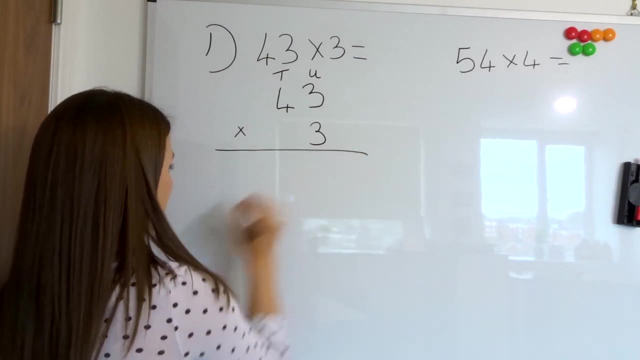 Then we're going to put a three underneath because we've got our tens column and our units column. Don't forget to put that multiplication there along the bottom and then leave a gap for two numbers and put another line. So we do start off with our units column. 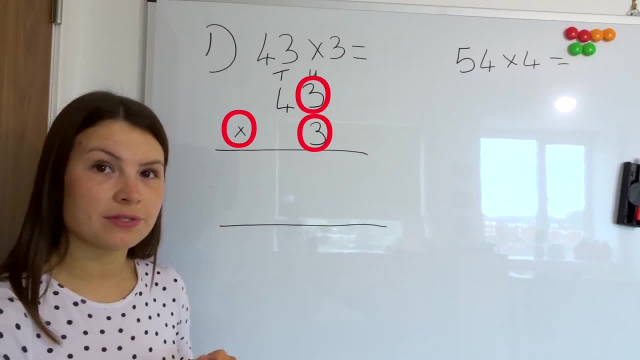 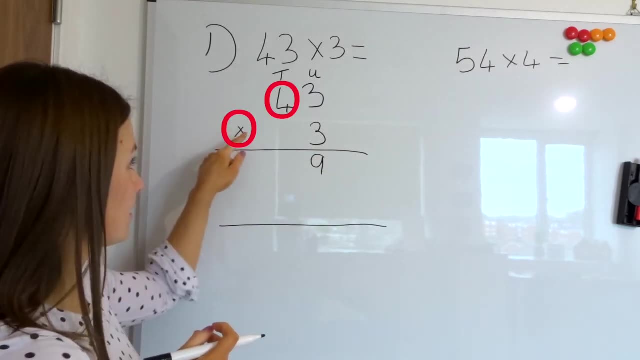 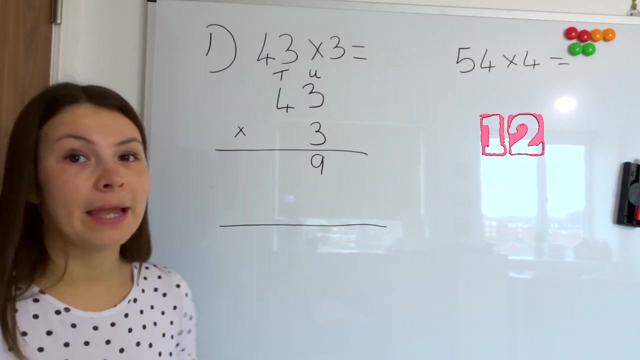 So three times three. What is three times three? That's right, Nine. Okay, Now we're going to do 40 times three, or four times three, and then make it 10 times bigger. So four times three is 12.. Make that 10 times bigger is 120. 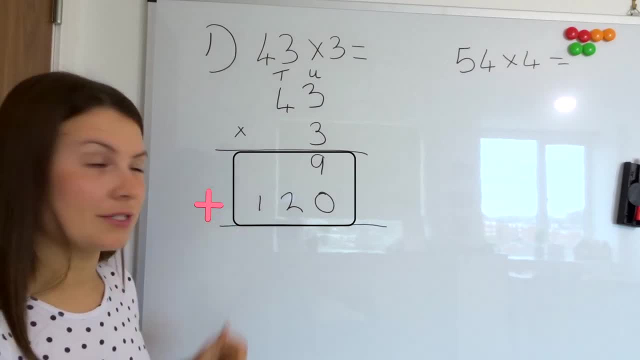 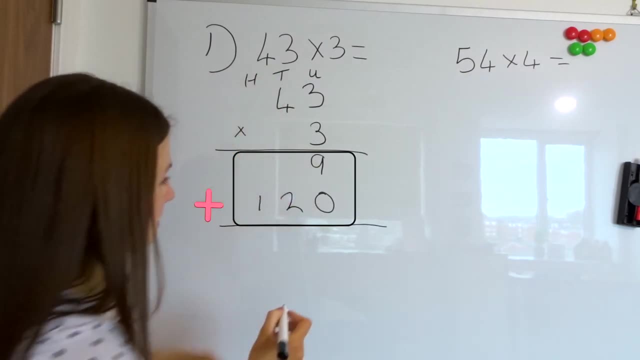 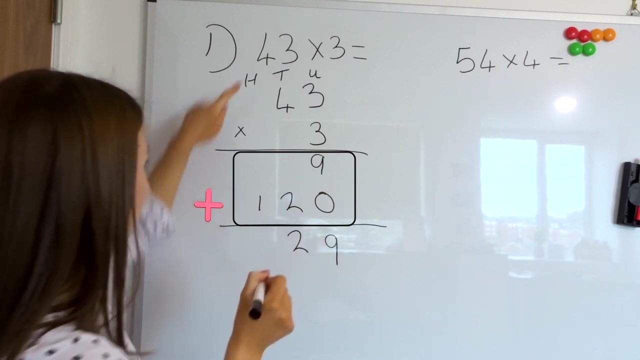 Fantastic. Now we need to add these two numbers together. Okay, So let's start off with my units. column Nine adds zero is nine. Tens: column Nothing add two is two. Hundreds. column Nothing add one is one, And your answer should be 129. 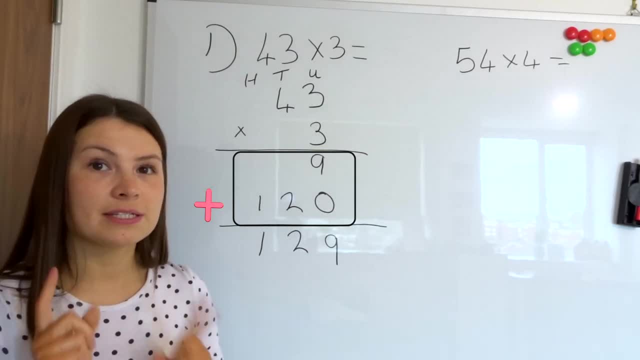 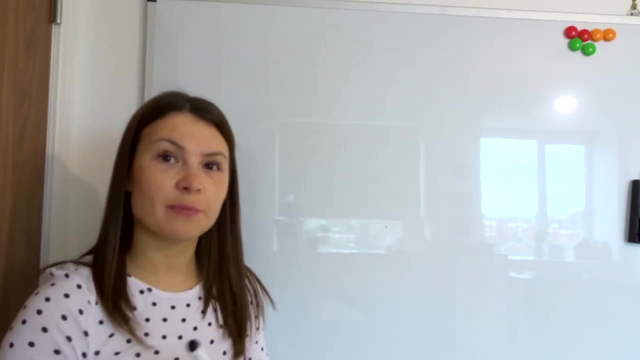 Big well done if you got that correct. If you didn't get that correct, just go back through where you made your mistake so that you can learn from it for the next one. Okay, So the next one we're going to look at is 54 times four. 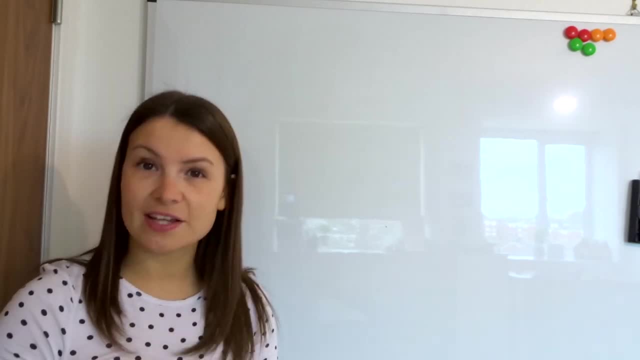 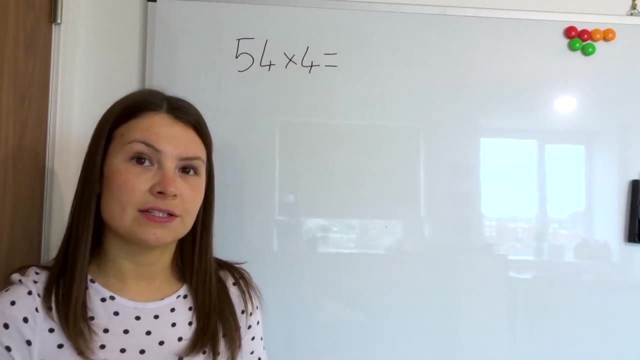 Now you should have already done this at home, So if you haven't already done this one, have a go at doing it now. Pause the video here. Okay, So 54 times four. So, just like with the other ones, we put the biggest number on the top. 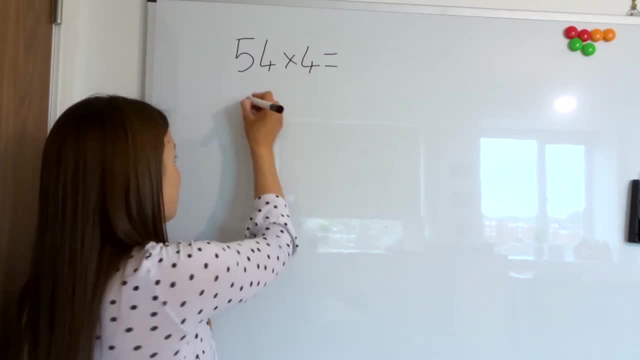 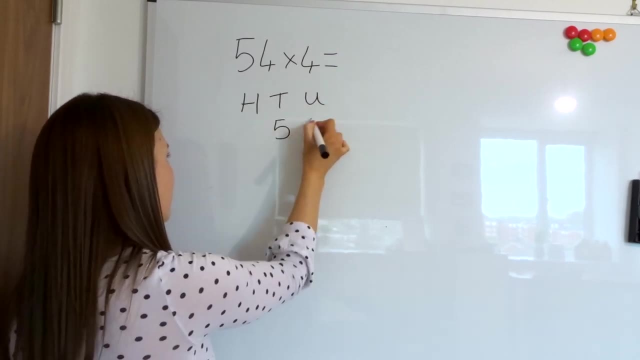 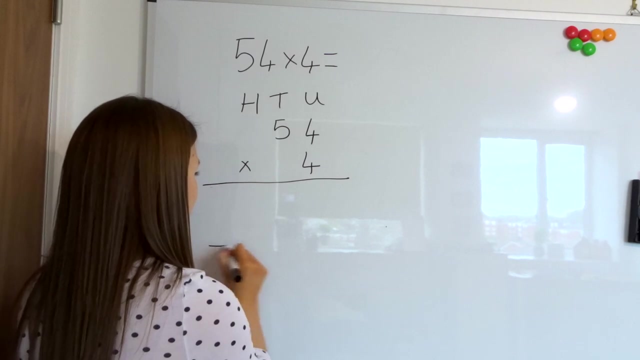 But before we do that, I'm actually going to put my hundreds, tens and units at the top. So 54 times four, One line here, Remember, leave a space for two numbers and the other line: Okay, Four times four. 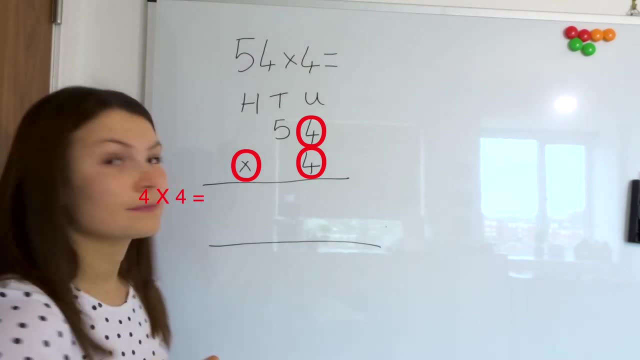 Four times four, It is 16.. Well done, Okay. And then we're doing 50 times four, Or five times four, and then making it ten times bigger. So five times four is 20.. Well done, Make it ten times bigger. 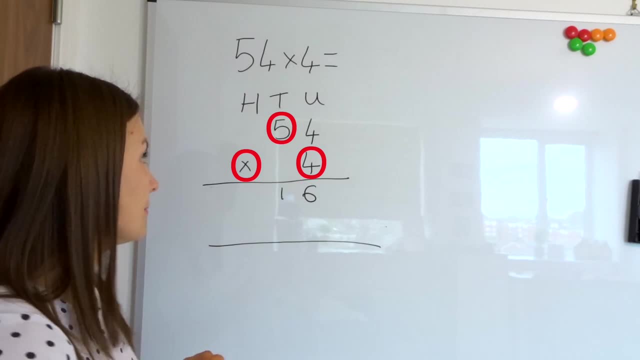 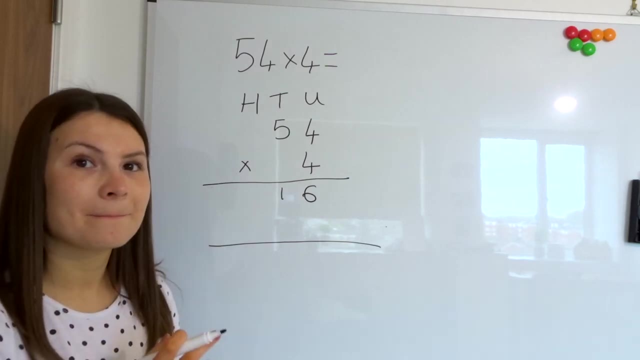 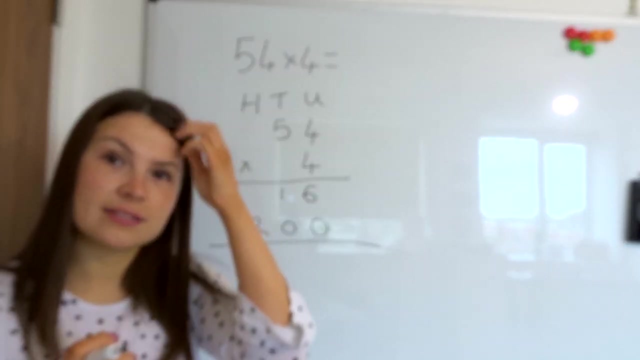 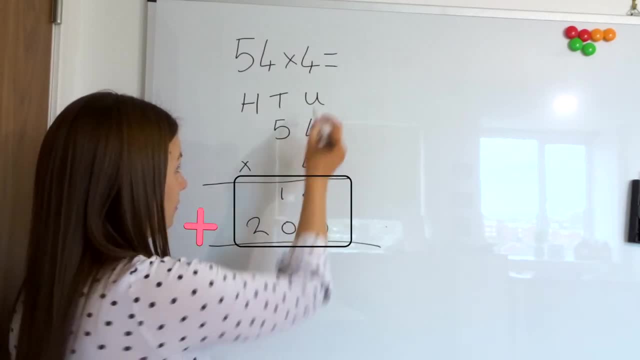 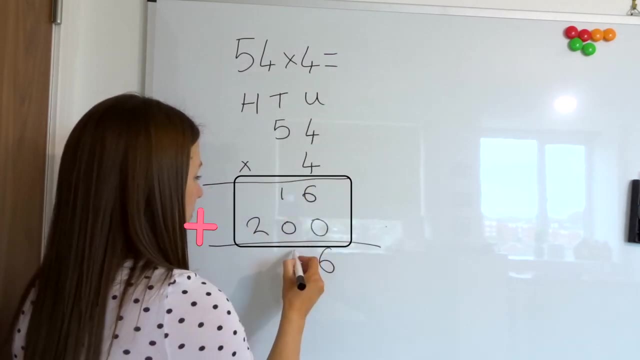 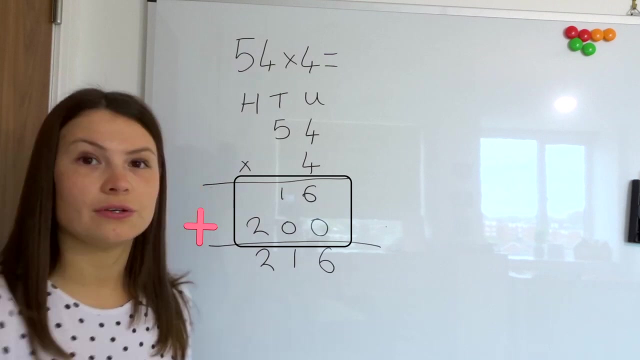 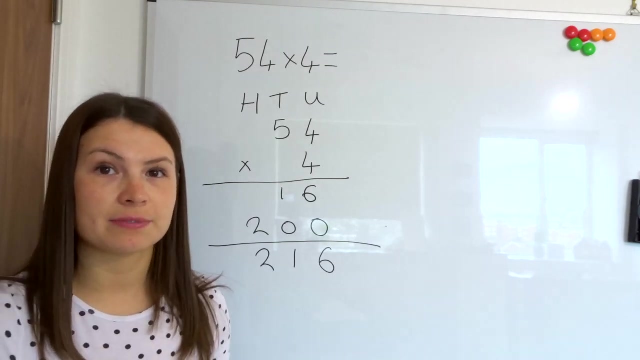 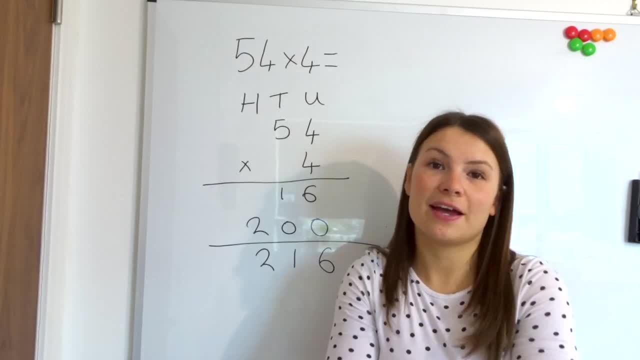 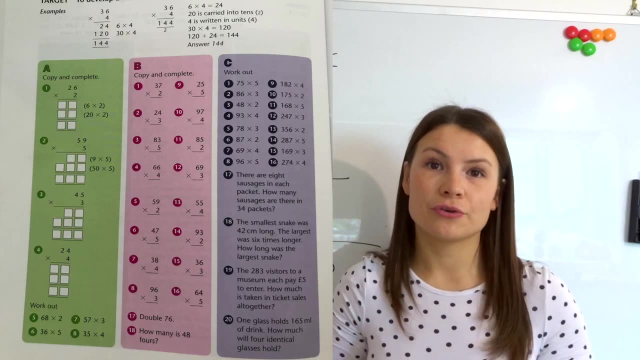 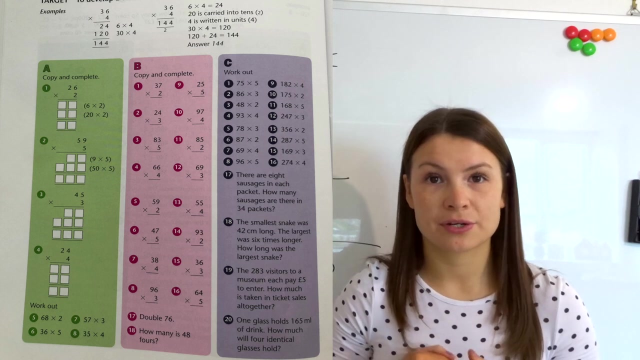 Okay, Okay, Okay, Okay of questions on written multiplication. have a go at doing these yourselves. if you need to go back and watch through the video, that is absolutely fine to remind yourself of the method. and if these questions are you are finding them a little bit tricky, perhaps ask an adult to write out some easier questions for 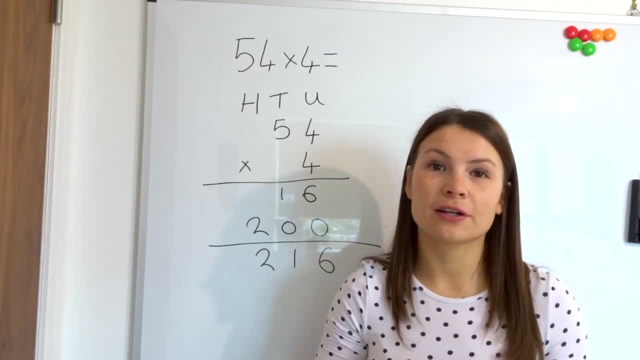 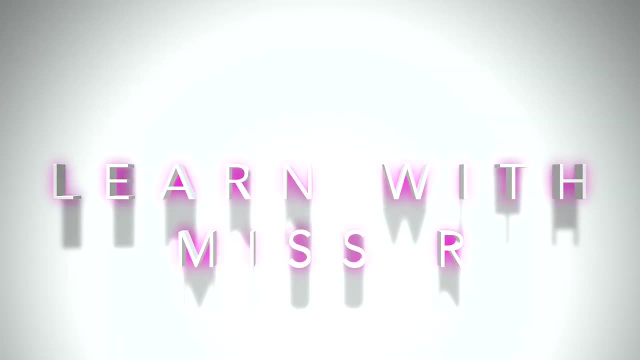 you on a piece of paper. I hope this has been really helpful and I hope you have learned lots from today and I will see you in the next video. you.